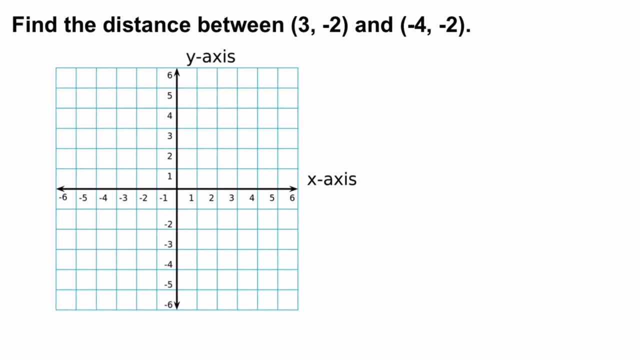 Find the distance between 3, negative 2 and negative 4, negative 2.. So I'm going to start at the origin. I'm going to go to the right 3 spaces and go down 2 spaces, That is, 3, negative 2.. 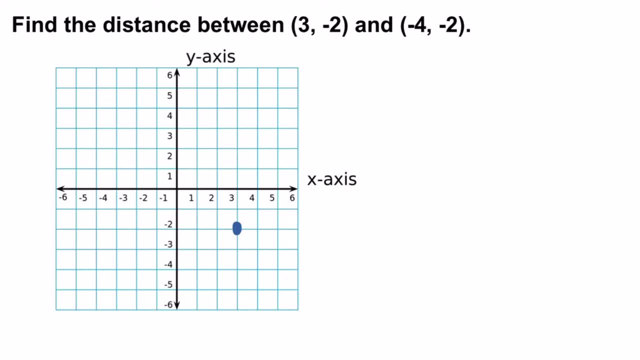 Now it says negative 4 and negative 2.. So I'm going to start at the origin, go to the left 4 spaces and then down 2.. And put a dot To find the distance I'm going to count from one dot to the next. 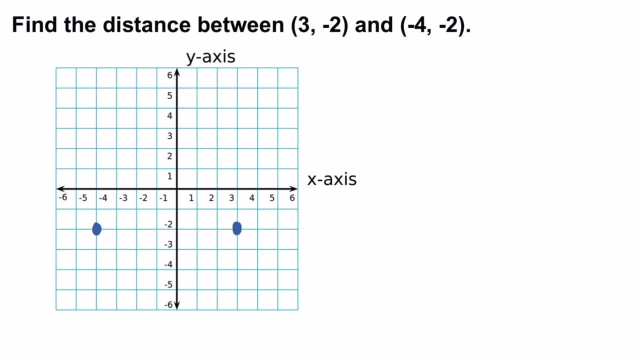 So I'm going to start here at the left, at negative 4, negative 2.. And then go to the right 3 spaces and go down 2.. And then go to 3, negative 2.. So this is 1,, 2,, 3,, 4,, 5,, 6,, 7.. 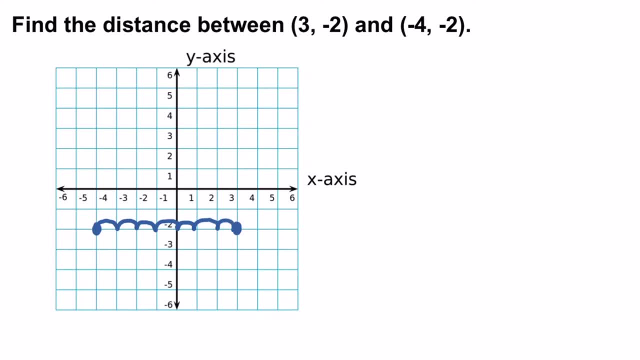 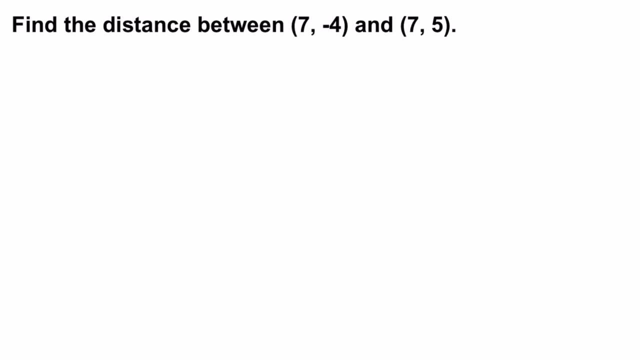 So the distance between 3, negative 2 and negative 4, negative 2 is 7 units. Okay, The next example: If you were not given a grid, you would need to figure out how to calculate the distance. So, if you notice, find the distance between 7, negative 4.. 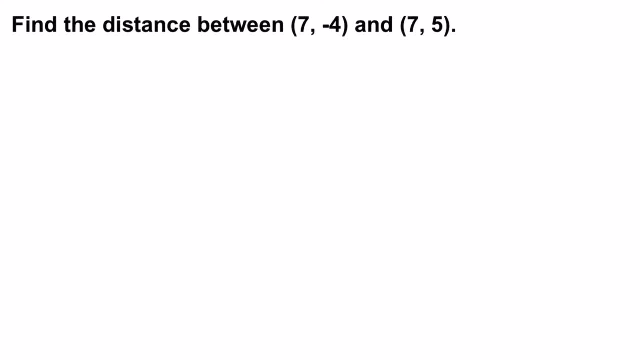 And 7, 5.. If you notice, the first two numbers are the same, or the X coordinates are the same. So all you have to calculate is the distance between the Y coordinates, which is negative 4 and 5.. So you will put negative 4 in the absolute value bars. 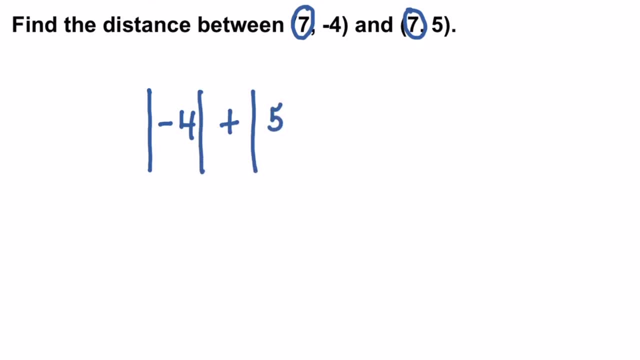 You're going to add it to the absolute value of 5.. And then you just rewrite the problem as positive 4 plus positive 5. And you get 9.. So the distance between 7, negative 4 and 7, 5 is 9 units. 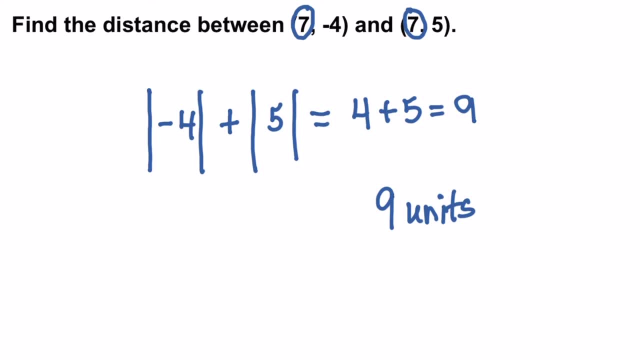 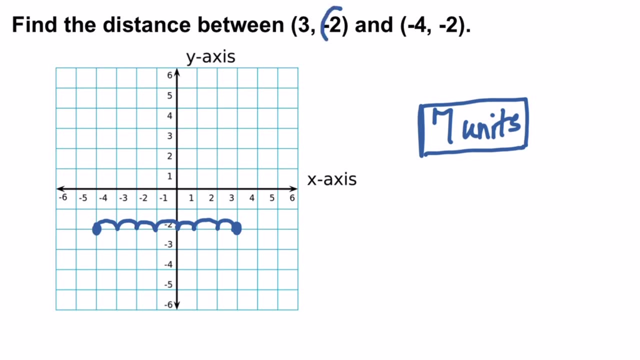 Okay, Now let's go back. just to make sure we are clear, We could have done the same thing here for this example. We see here that the Y coordinates are the same, So in order to calculate the distance, I can do the same thing. 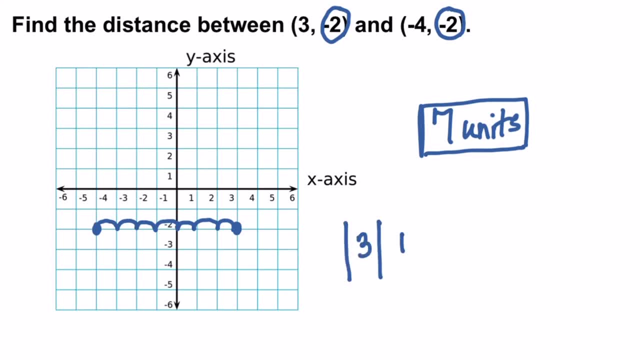 I can say 3,, the absolute value of 3.. Plus the absolute value of 9.. Negative 4.. And then I rewrite the problem as both positive numbers, 3 plus 4. And I get 7 again Again. let's go back to the first example.